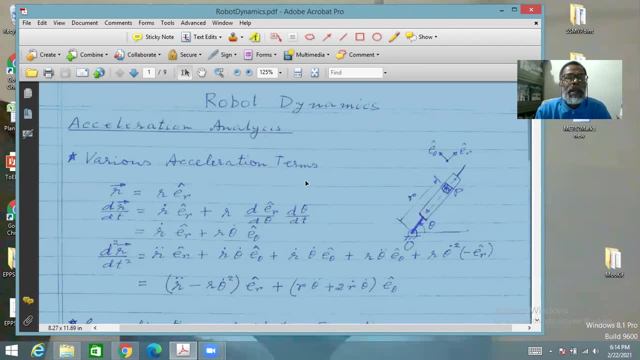 from the velocity analysis which we have already covered. But to begin fresh, let me first show you the origin of various acceleration terms. For that, consider this simple system of one link, pivoted here at point O, which is fixed for the time being. 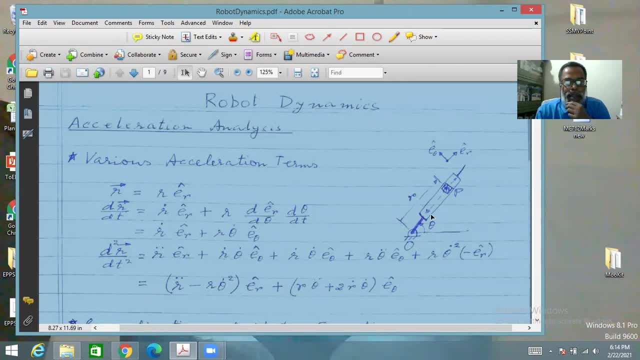 And in this link there is a slot, radial slot, in which there is a slider. So as the link rotates about O, the slider can slide along the slot. So let us find out the acceleration of this slider point P, reference point of the slider P. So start from position. 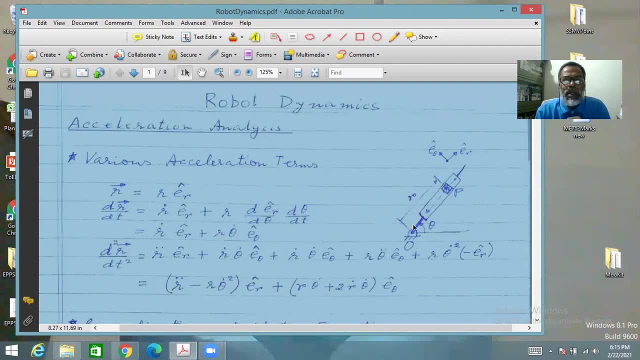 So position will be: magnitude r, direction the unit vector along r. So that is this. Now, when you try to find out the velocity of point P, then you basically differentiate it with respect to time, And this is a product in which the magnitude as well as. 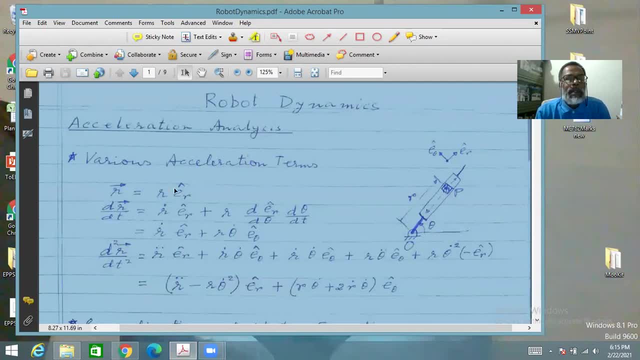 the direction can change with time, So use the product rule of differentiation, Derivative of this, into this, plus this held into derivative of this. So this is r times derivative of er. Now you see, er is the unit vector in this direction. 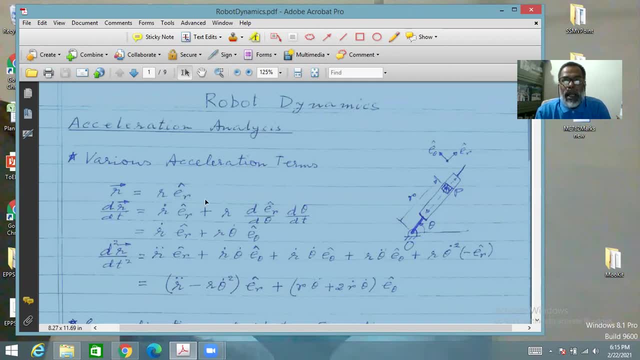 Now, as motion takes place, the link rotates, So er will change its direction. It will change its direction from this to this. This direction, which is perpendicular to er, is denoted as e theta, Because if you keep r as constant and change theta, then this is the direction in which it moves. 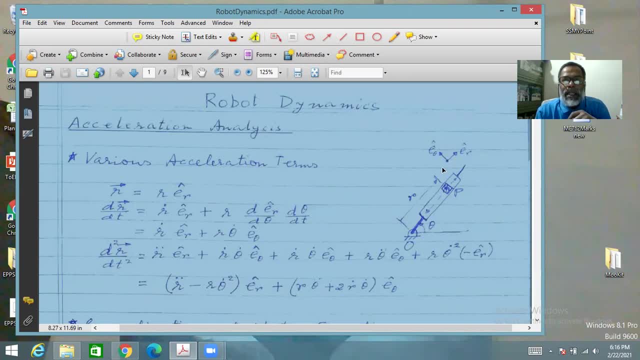 OK, So the unit vector in this direction, as it changes direction, does not change magnitude because later also it remains a unit vector. So you know that the rate of change of a unit vector with respect to the angular motion, theta, is the unit vector. 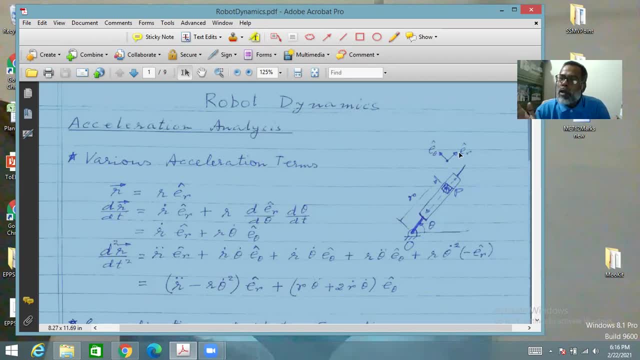 that русin terms, that does not have belt on it. So sometimes in this movement that來到 is an upper bound, that is, does not play a part of this differential model. Another point: Yay, We made it Okay. 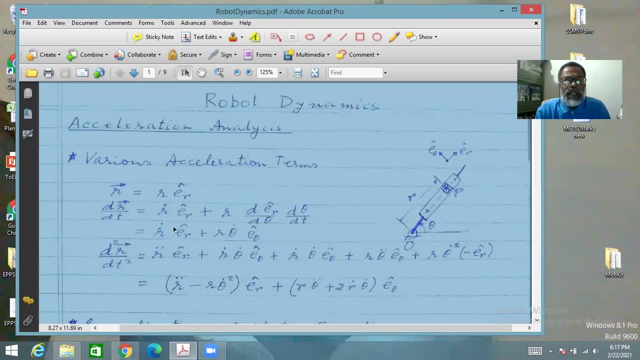 That was interesting. That was interesting, See theε. And finally, I hope you have any other questions in this. All right, Thank you, bye, Bye. in which this is the radial component and this is the transverse component. you know that. so this is. 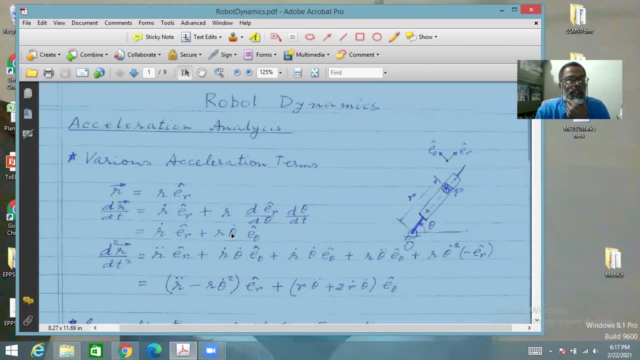 r dot radial component. this is omega cross r transverse component. now to find the acceleration of p. you differentiate this with respect to time. so again, product rule. so derivative of this, r double dot into this as it is, plus this as it is, into derivative of this, which we have already seen. 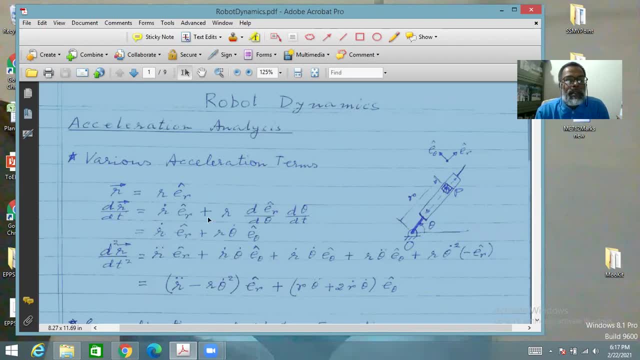 theta dot into e theta plus. now come to here, come to this term. this is a product of three things, right? so there will be three parts in the derivative r dot, theta dot, e theta. this one has come from here, from here we get this. so then r theta double dot, e theta here and finally r theta dot into derivative of this. 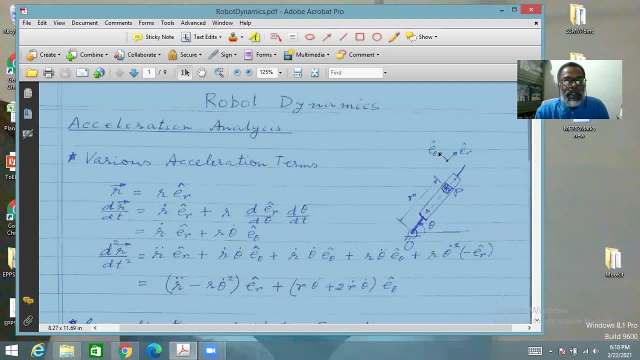 so e theta. when you differentiate it with respect to time, you say differentiate it with respect to theta and then multiply with d, theta by dt. so as you differentiate this unit vector with respect to theta, it turns further by another right angle, becoming negative of er. fine, so that is here. 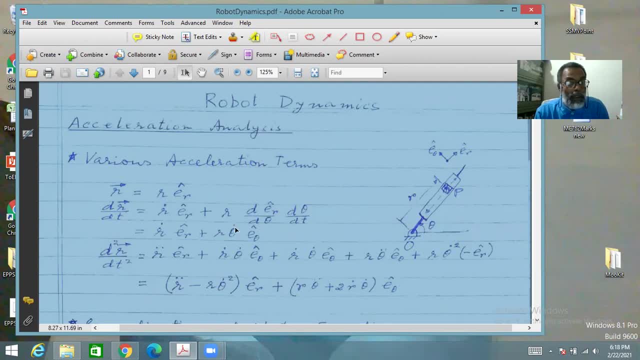 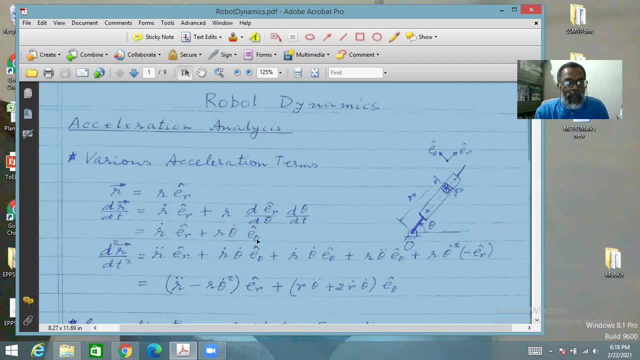 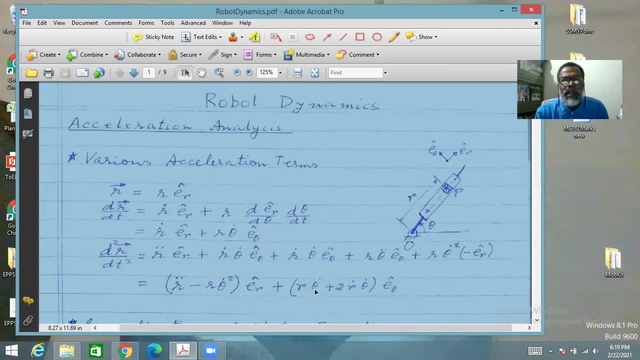 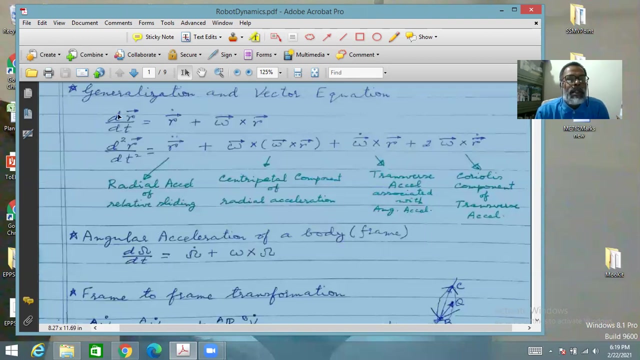 direction. you get this term which is here, and you get these two terms equal. so twice that fine. so this is what the acceleration of this point P is now in vector notation. let us jot them down term by term, so dr by dt. is this which we already already saw and discussed, and this one has four terms: this, this, this. 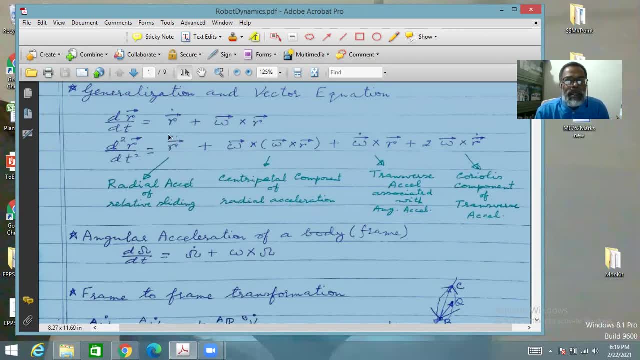 and this. so this term is the radial acceleration of relative sliding in the sort. okay, this is the centripetal component of radial acceleration. okay, this is the centripetal component of radial acceleration. this alpha cross r is the transverse acceleration associated with angular acceleration: Angular 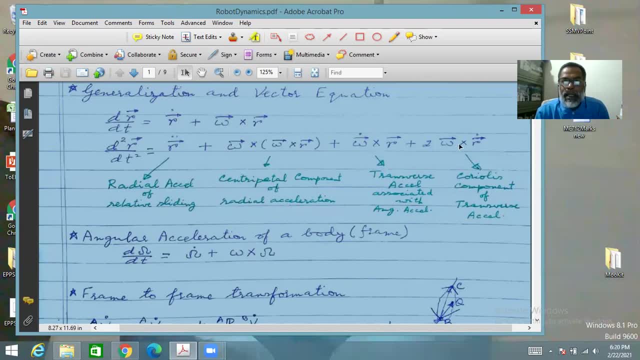 acceleration of the link is this, And this is the Coriolis component of transverse acceleration. Transverse acceleration has a funny component called Coriolis component, which is always associated with sliding motion in a rotating body. So that is twice omega cross sliding. 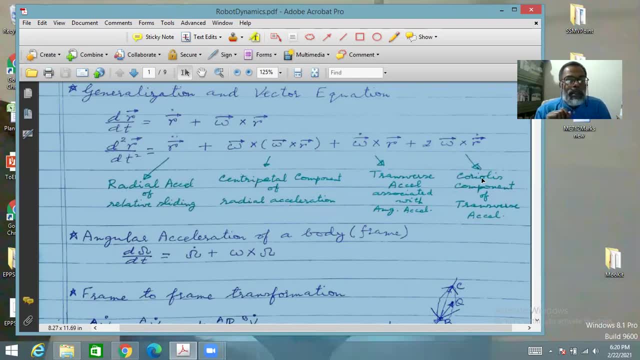 velocity. Fine, Now, till this point, the point O was fixed. If O had its own acceleration, then, apart from these four terms of acceleration, the acceleration of point O also would get added to the acceleration of point P. Okay, Now, all this is regarding the acceleration. 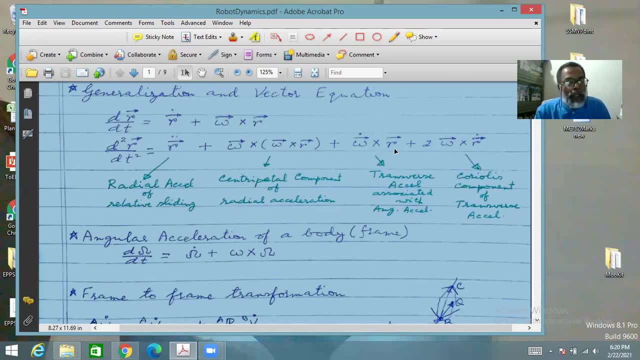 of a point. linear acceleration of a point, Angular acceleration of a body- to find out that You differentiate this directly- and plus omega, this small omega, cross capital, omega. Well, capital omega is the angular velocity of the body, of which angular acceleration. 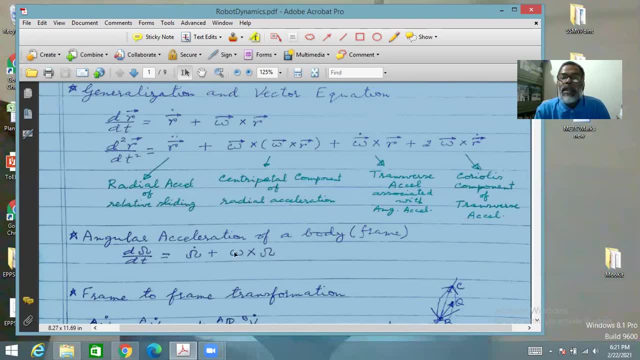 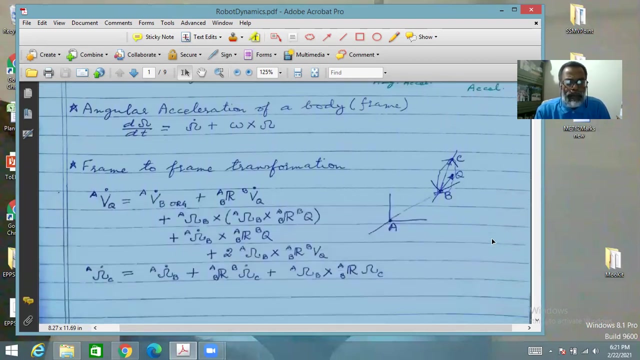 is sought, And this omega is the angular acceleration of the frame in which that description of the body is there. Okay, This term is one important term which you have to keep in mind, not forget. Okay, So, based on this, when we conduct frame-to-frame transformations, then our intention typically 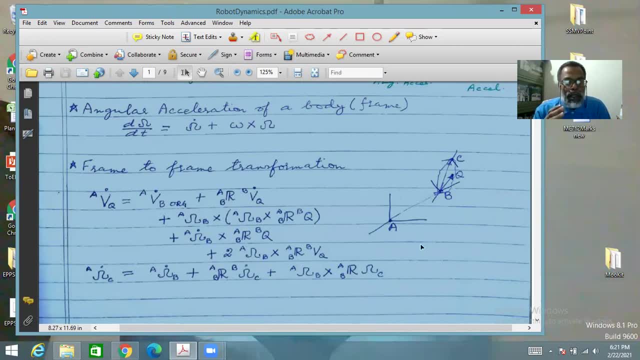 would be to convert linear acceleration of points and angular acceleration of frames or bodies which are available in one frame. This brings us back to the theory of linear acceleration of point P, so we can get another frame B to another frame A. Okay, smoothly, smoothly, smoothly, All right. 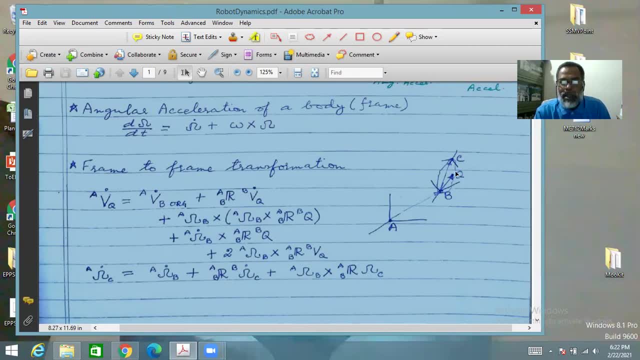 That is, in frame B, the position, acceleration, velocity, acceleration of Q, is are described, are available, and orientation, angular velocity and angular acceleration of a frame C is available And we would like to get them in this frame A. Okay, So for that, first for the point. linear acceleration of point P. okay, All right. Now this is a linear-anterior relationship. There are three points, B and B, There are four points C and there are three points D. Now what do we call these three points? 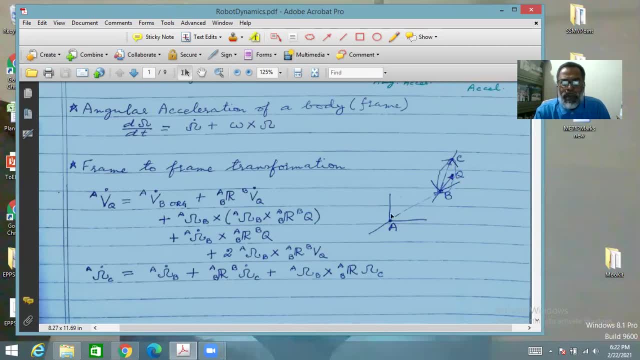 linear acceleration, linear acceleration of point Q in frame A. So for that we need to find out, we need to include first the linear acceleration of point B and then in frame B whatever is available of point Q, those four terms, okay. So first in frame A the 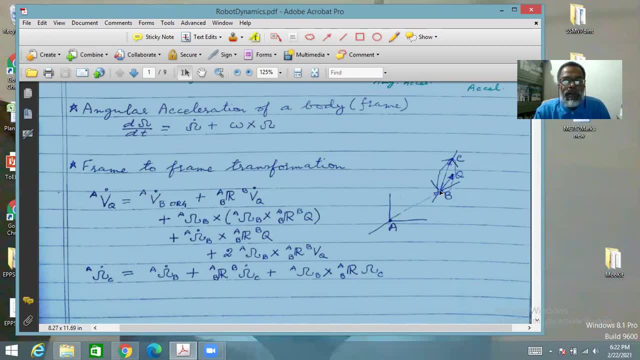 acceleration of the origin of frame B, that is this VB, dot or VB or G dot, plus now the four terms. This is the straightforward R double dot term. okay, This is basically to convert this vector to the frame A. okay, Then the centripetal term. this is the direct. 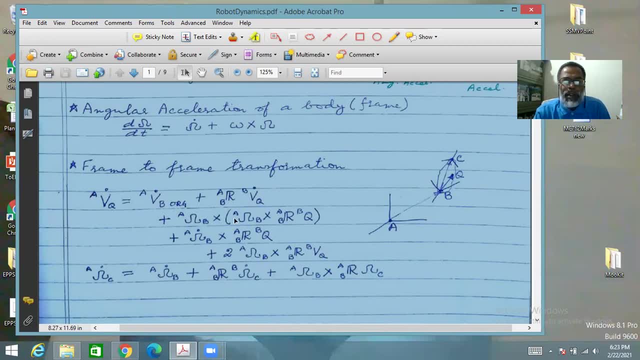 radial acceleration. This is the centripetal acceleration. omega cross, omega cross. Now these two omegas are omegas of omega, of B in A right. So this vector also has to be expressed in A. so that is why this multiplication is here. Otherwise Q is just the position in frame. 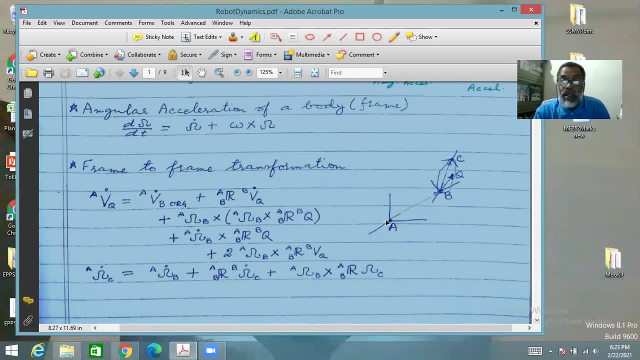 B. okay, So that has been converted to this in this basis. okay, by this orientation matrix. So this is the centripetal combination component of the acceleration of Q And then the direct angular acceleration that is because of the angular acceleration of frame B. so alpha cross, R, R is this vector, Q in frame. 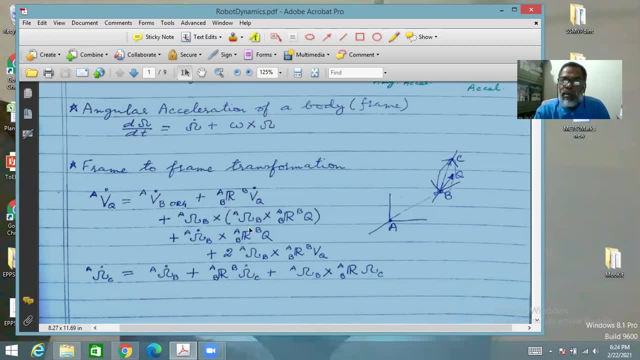 B converted to this because for cross multiplication you need both the vectors in the same frame, in the same basis, plus the coriolis component, As usual, twice omega, cross the sliding velocity, the relative velocity, and convert it to the proper frame. So this is the transformation. 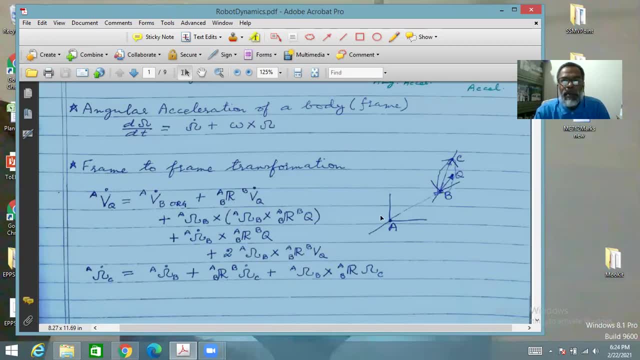 of the linear acceleration of Q from frame B to frame A. Now for angular acceleration of a frame described in C. you use that Three terms will come. One is the angular acceleration of this frame itself, plus two terms. One is the direct angular acceleration of this, which is this converted to the frame. 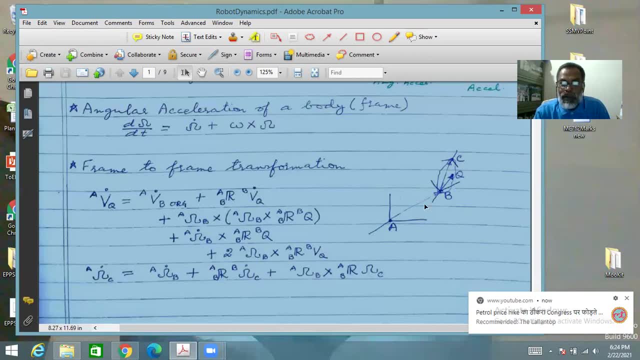 A plus omega of this, cross omega of this brought to the same frame. So these things, when we do recursively from frame 0, which is fixed, to frame 1, to 2, to 3, and so on, so on, we describe the acceleration quantities of all the frames, all the relevant points. 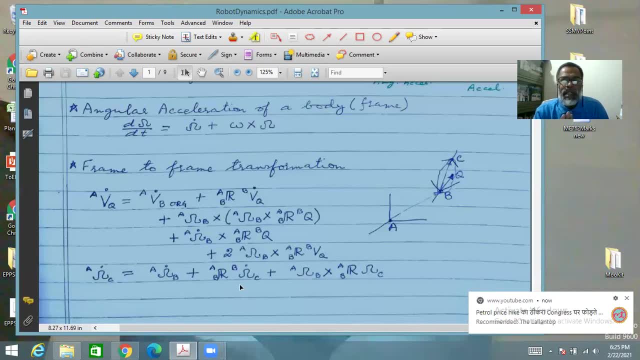 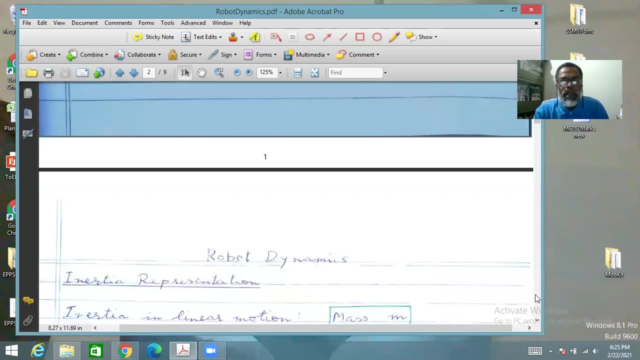 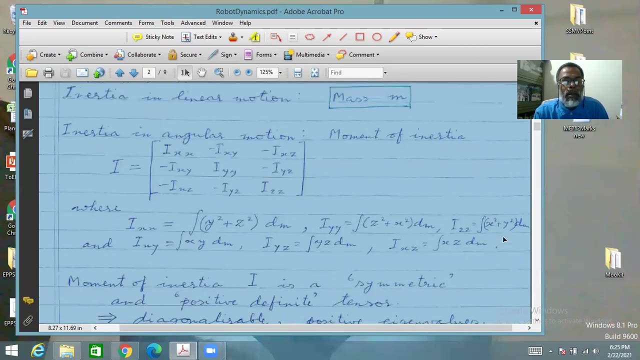 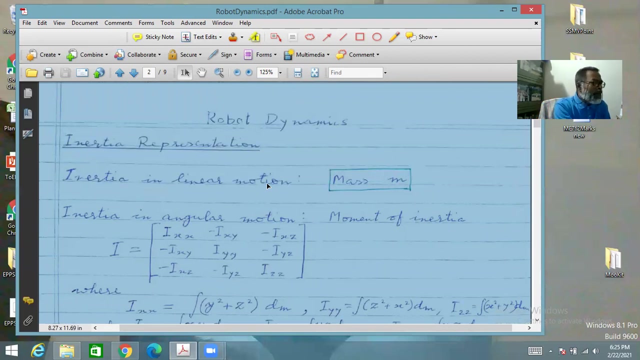 on the way. So this is regarding acceleration analysis. Now let us come to inertia distribution – inertia representation. Inertia in linear motion is just mass. Inertia in angular motion is given by moment of inertia, which is this: Tensors, symmetric tensor, where the definition of this, Ixx, etc. is this And this you. 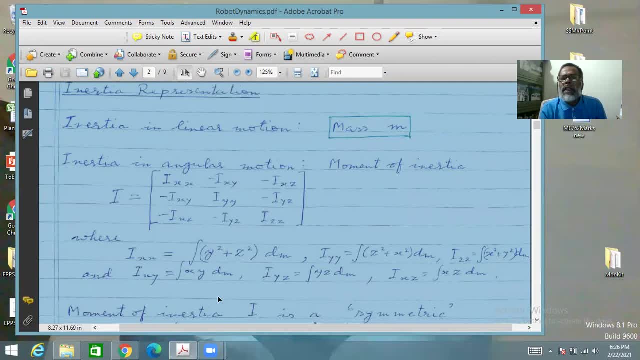 can find out from the straightforward definition of single-axis moment of inertia. So from the x-axis, this is a distance square, y square plus z square, into whatever little mass is sitting at that y z location. So that is this. And when such little masses, the rotational inertia of such little masses. 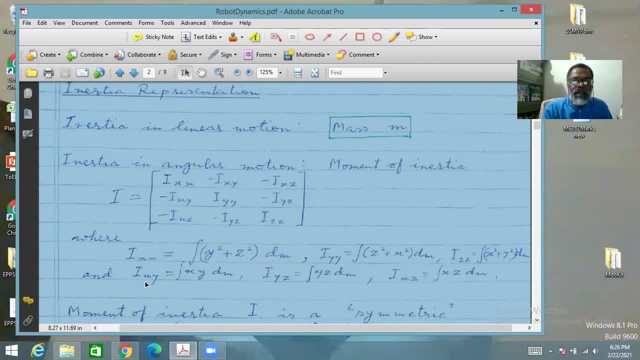 is summed up, then you have this- And this is the product of inertia- defined like this: So all the six terms, actually, out of the nine terms, only six terms are independent, because this is symmetric. So the definitions of this you have. So moments of inertia and 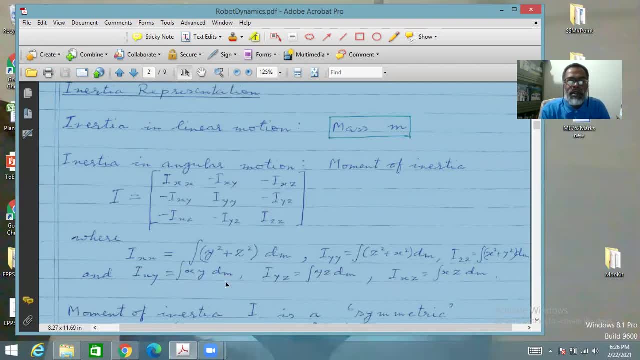 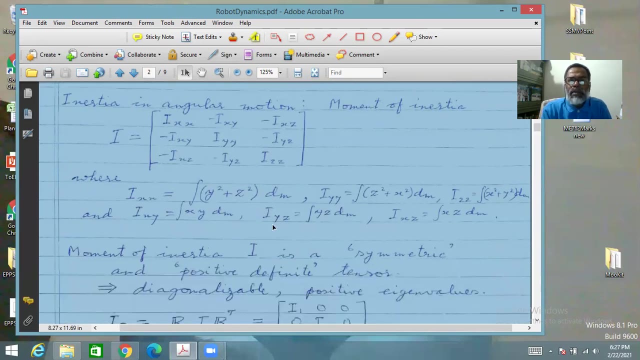 products of inertia. Single-axis moments of inertia and products of inertia. So the products of inertia assembled together. like this you get the moment of inertia of the body. And moment of inertia is a symmetric, positive definite matrix or positive definite tensor, Symmetric by definition, positive definite by the physics of it. No body can. 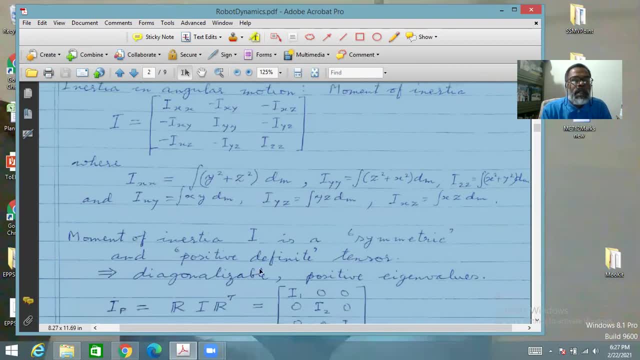 have negative inertia. you see, So that is the physics of it. So since it is symmetric, the tensor is diagonalizable and since it is positive, definite, it is constant. So there is an inverse of the inertia. So here you can see the inertia, moment of inertia. 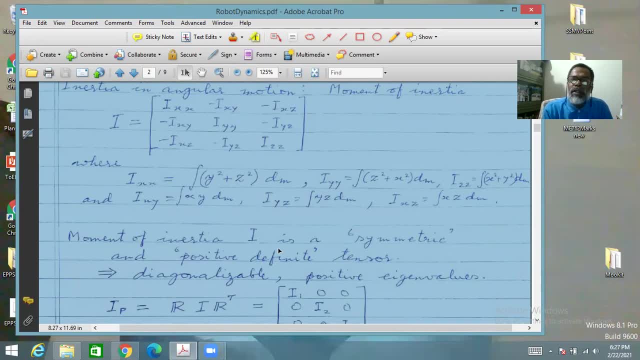 of the body, So that is in terms of the inertia, moment of inertia. This is an inverse or aНуxial definite after diagonalization. the diagonal entries will all turn out to be positive, that is, all eigenvalues will be positive. fine, so symmetric matrices are diagonalizable with. 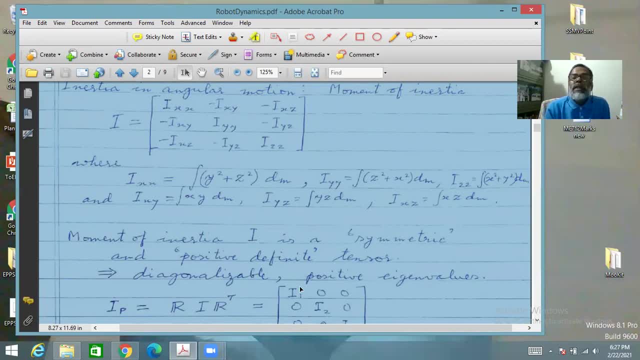 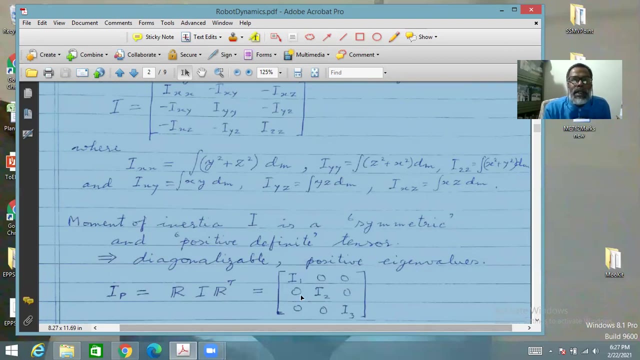 respect to orthogonal similarity transformations. okay, that means finding an orientation matrix r, appropriate orientation matrix r. you can diagonalize them and get it like this: okay, so actually, apart from mass, these three quantities are the real physical property of the body, the inertia property of the body. earlier nine numbers or six independent numbers that we had. 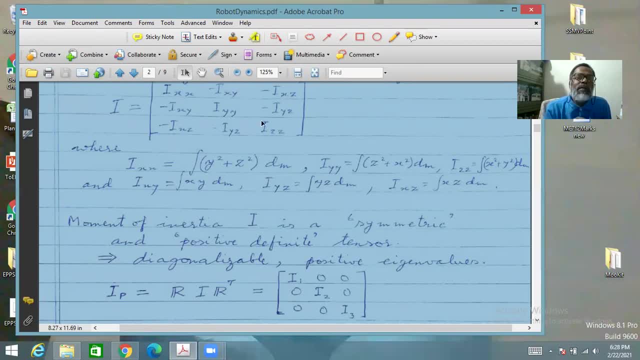 here. they were a combination of the inertia property of the body and the axis chosen. okay. now, when you do this, it is important that you have this about a frame of reference. okay, in a set of axes passing through the center of mass. okay, so you have this. 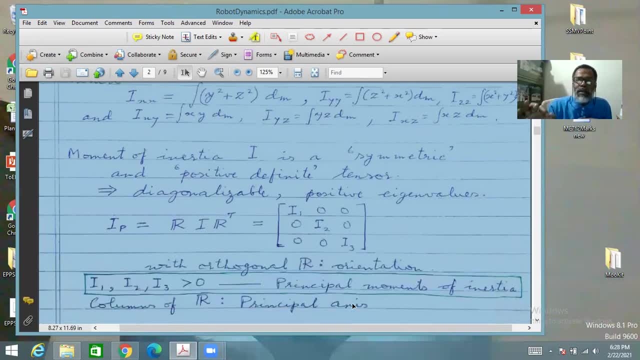 so m, i1, i2, i3, that is mass. then moment of inertia of the body about three mutually perpendicular axis which happen to be principal axis of that body. okay, so these four are actually inertia properties of the body. for every digit body you have a set of principal axes passing. 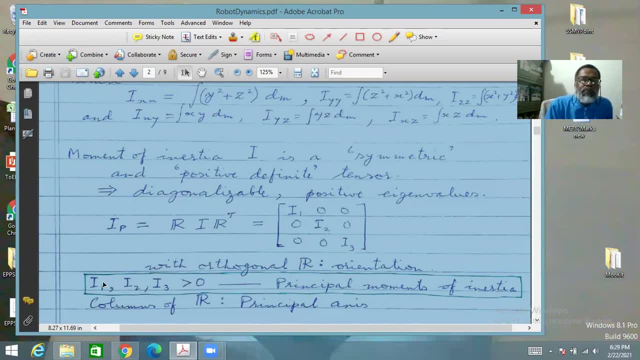 through the center of mass. okay so, but though these are the actual physical properties, if we are working in a different frame of reference, we may have to think about the physical properties of the body and we may have to convert, i mean, we may have to actually operate with those six numbers. 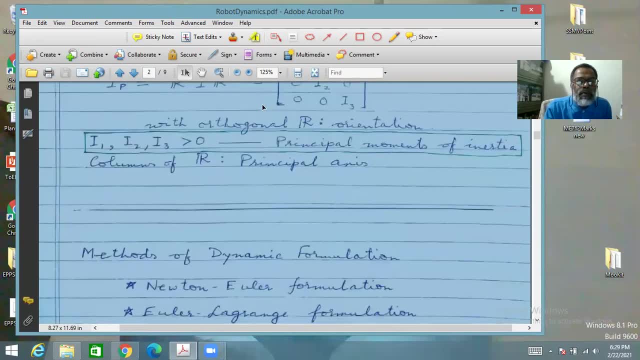 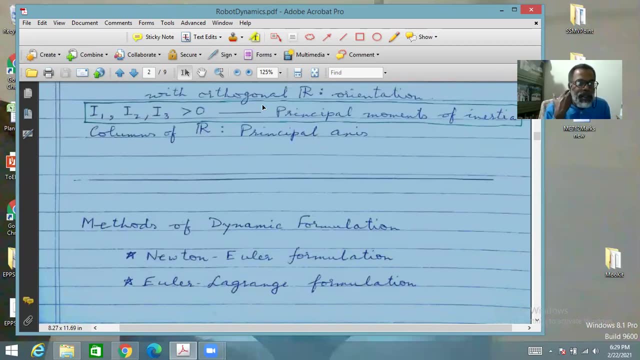 okay, fine, now, having covered the background of acceleration analysis and inertia representation, we are now in a position to talk about dynamic formulation of robot manipulators. there are two standard methods of dynamic formulation. one is Newton-Euler formulation and the other is Euler-Lagrange formulation. 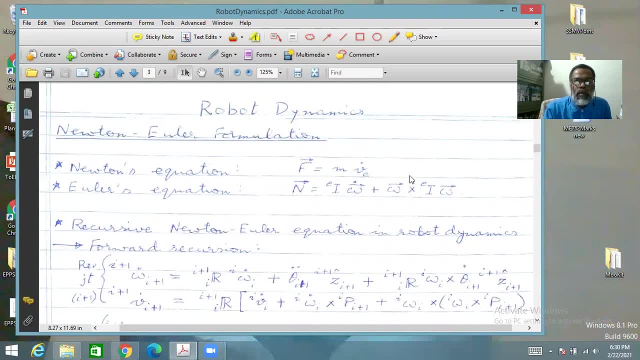 so first we talk about the Euler formula. so if I have a formula n equal to n times 1, and then I am going to call this formula c and the integration of the formula c into the formula c. so these are the very first and the fundamental steps. 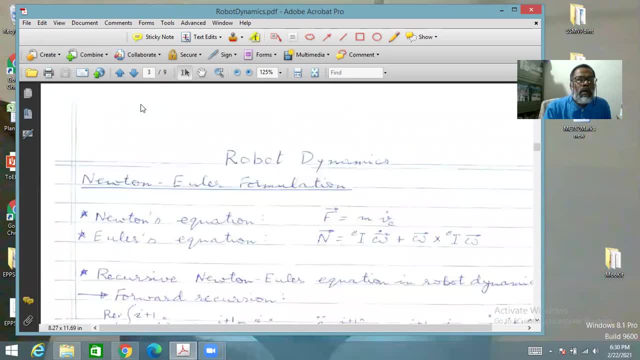 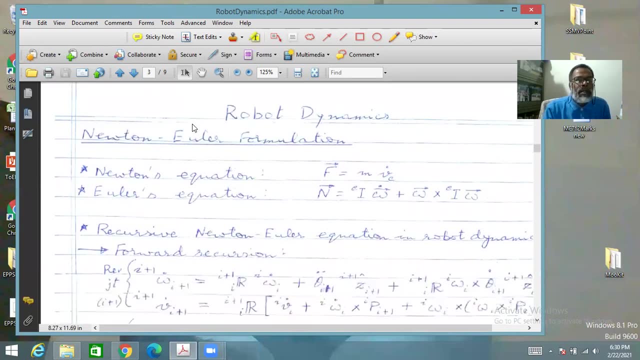 so, when we talk about the integration of the formula c into the formula c, we are going to be talking about the neutral formulation, we are going to be talking about the type of formulation that is equal to the terms of the formula c. in order to explain this problem, 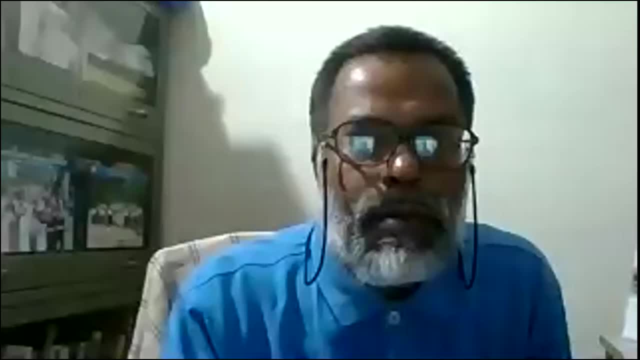 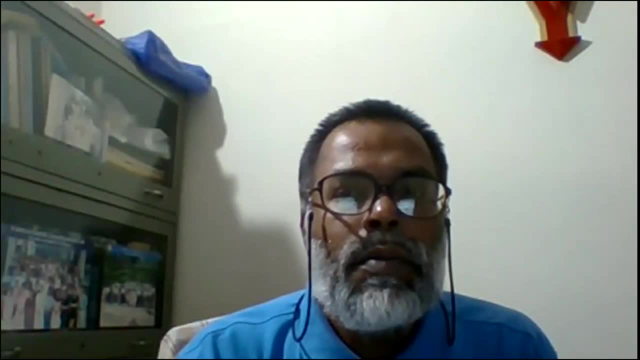 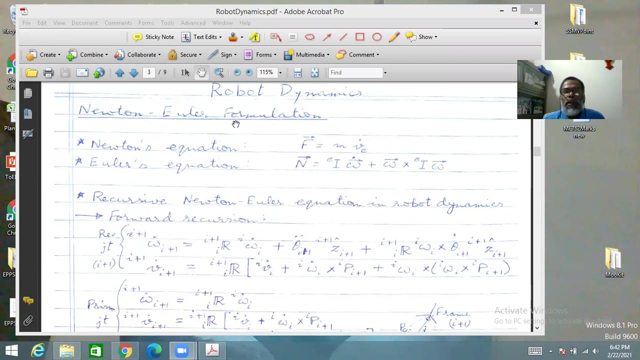 Yes, So in Newton Euler formulation we directly use the Newton's equation for linear motion and Euler's equation for angular motion. Euler's equation is actually not Euler's law, as Newton's equation is Newton's second law, because Euler's equation gets arrived at when. 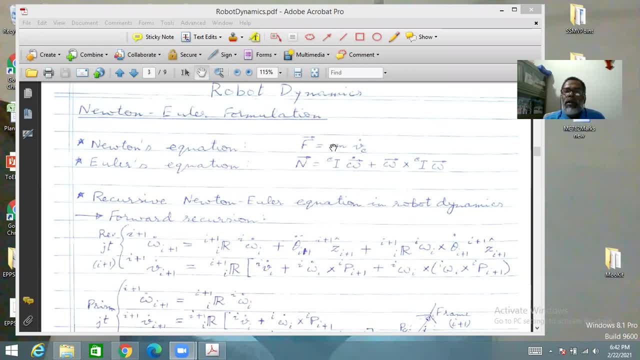 you apply Newton's second law over all the little particles of a rigid body and sum them together, Then you basically get this- So Newton's second law- all of you know that the total vector force on a body is equal to mass- into acceleration of its center of. 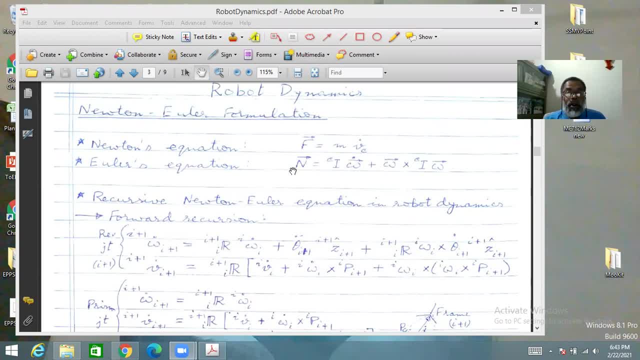 mass. The Euler's equation is similarly total vector moment on a rigid body is the moment of inertia of the body about a frame of reference And we interpret the method for this as the initial of Euler's equation. So we have this Euler's equation for the vector of the. 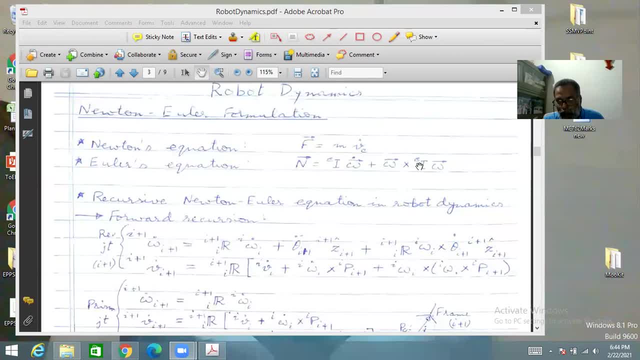 moment on a rigid body- I will put it in the description, And that is the original time, current which the vector is passing through- or with the origin at the center of mass, into angular acceleration Plus omega cross, that same moment of inertia times, omega. So this vector is multiplied with this matrix and then whatever. 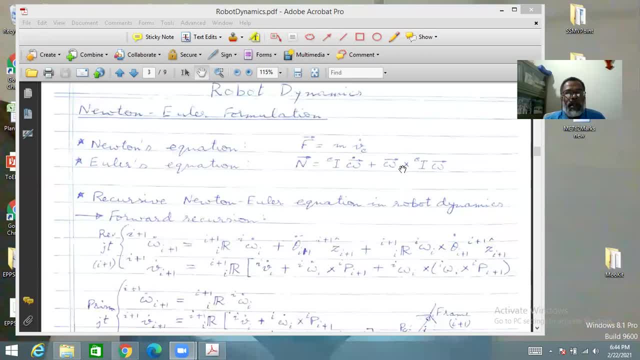 vector comes, you cross, multiply omega with that. So students often forget to include this term. because in planar motion only this term is there. okay so, but you have to include this, because now we are talking about spatial 3d motion. okay so the neutral euler equation in robot dynamics is basically recursive forward recursion for. 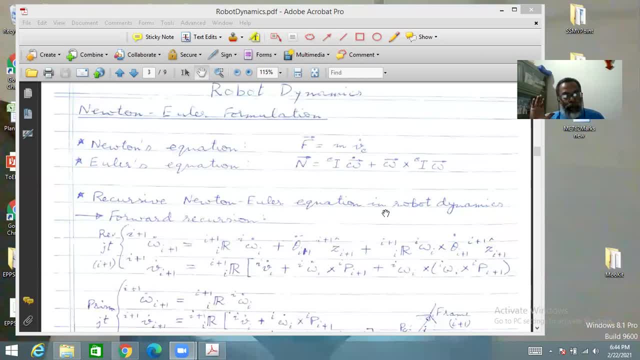 acceleration using the terms that we studied just a few minutes back. for the acceleration analysis and then for forces, we conduct backward regression from n to zero, the way we studied the static force transformation from the hand to the base. okay, so the forward recursion, the angular acceleration of i plus. 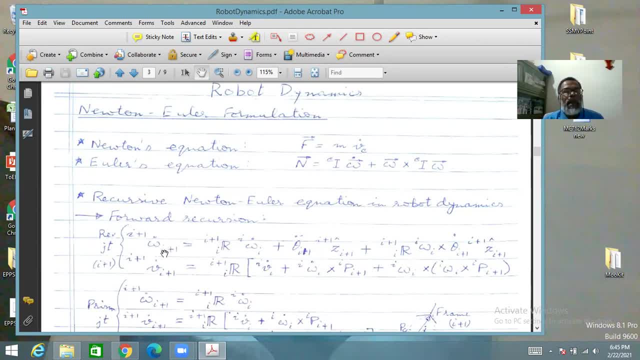 polarization x and the né starting time of i plus Bali. 1th frame of reference is the angular acceleration of the ith frame of reference converted to the proper basis, plus two terms. one is the direct angular acceleration term. now this is for evaluate joint, so the i plus 1th joint is evaluate, so it can have a an angular. 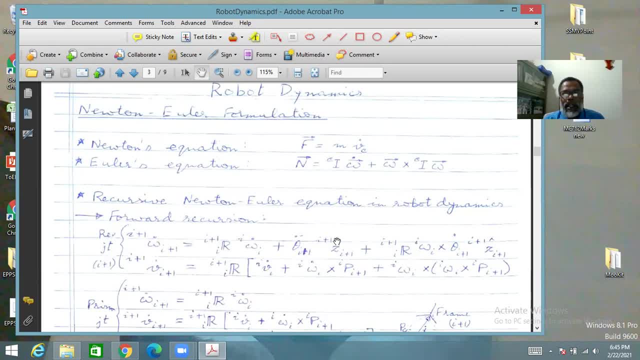 acceleration of the joint, so that angular acceleration into its that magnitude, into unit vector. this is essentially 0, 0, 1, okay, in i plus 1th frame itself, plus omega cross, omega of i cross, the omega, omega of i plus 1, converted to the proper basis. okay, so now. 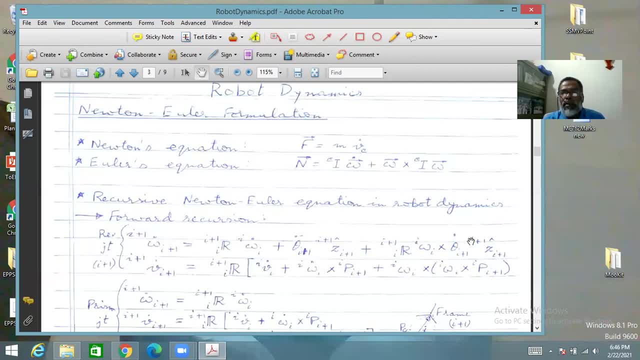 this has to be have to be converted to i plus 1, because this vector to begin with is i plus 1 and as the result is finally short in i plus 1, so that is how we will leave it. so this converts the angular acceleration of the i plus 1th frame. expresses it okay, so 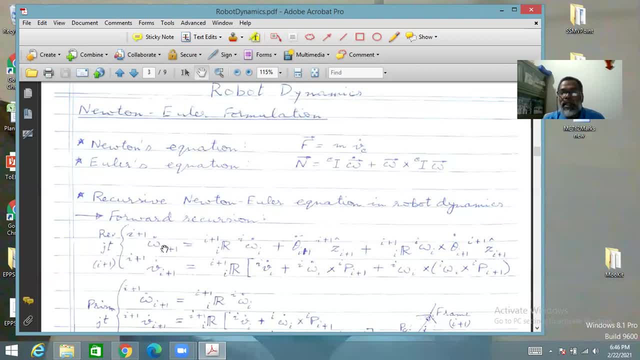 this puts the complete angular acceleration of the i plus 1th frame express in its own basis, including the earlier frame plus the i plus 1th frame. so that is how we will leave this front and end of this data. why is this thing called angular acceleration? because 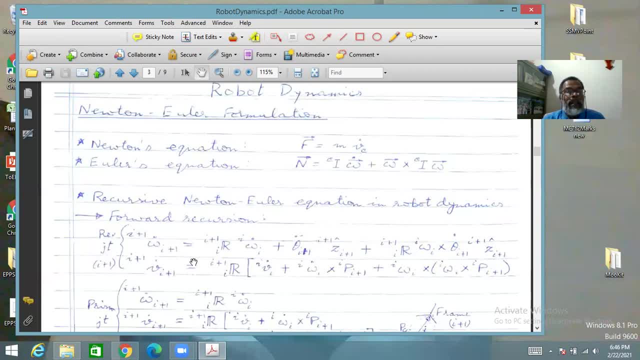 this is an odd 부분 of an arc. the in Austria and in India勾 these squares to be straight anywhere. they be in the same direction also, but for that they represent only one meter and i cross, say, with that first curve about 676.32, but this time it is one meter on. 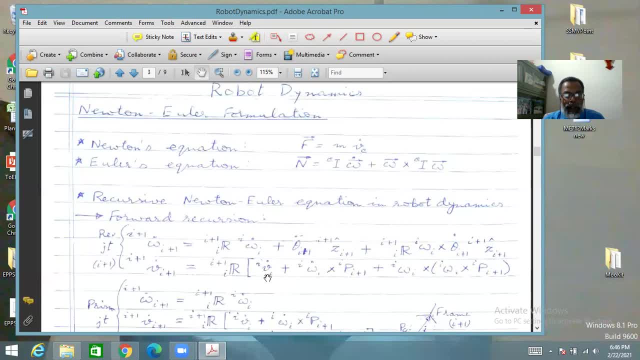 So approximately how much space? or it forhertz define the wzglhind that difference? the отправge, the easier term, is actually one meter, so it can maybe define and shouldn't say that truth either. some extra change helped to, given the rectangle function is limited and positive. right it was to define. it's given very fairly. because one second, because we will improve the foruffs. sorry so, without anything else before this. on to the durини too- not that I'm not saying much- which simply seek a cubic series, this method, so with related, i forhammer. 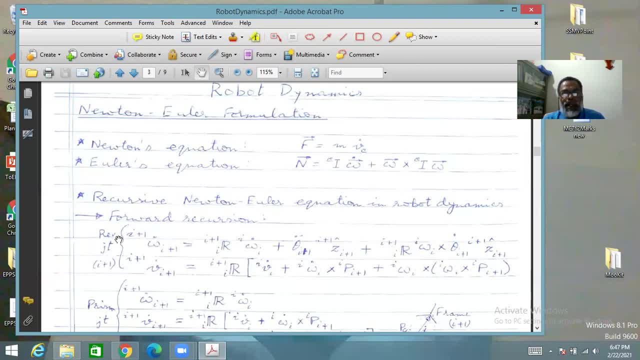 and curves. further meaning instead of dengan and spin right here the. that will be that climate this假 allowed. So r double dot term is missing and the Coriolis term is also missing because r dot is also 0.. So the remaining two terms, alpha plus r direct angular acceleration term. 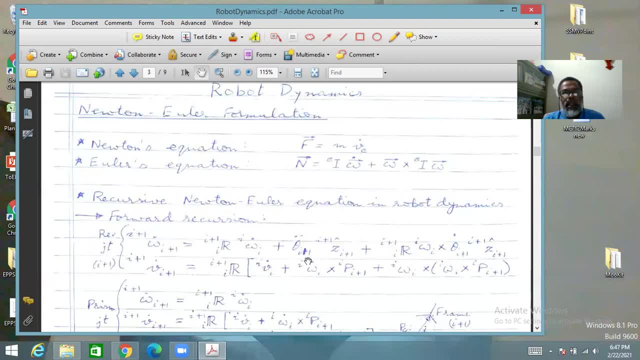 and the centripetal term omega cross, omega cross, r. So those two terms remain and this entire vector is then finally converted to the i plus 1th frame, because that is the basis in which we need to answer, because these things will later be used for the other one. Now, 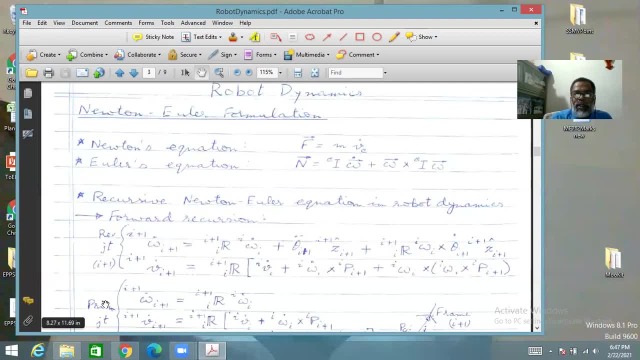 if the i plus 1th joint is not a reversed joint, if it is prismatic joint, then the angular acceleration of the i-th joint and i plus 1-th joint will be same, because in between no rotation is allowed. Now here the linear velocity component is: 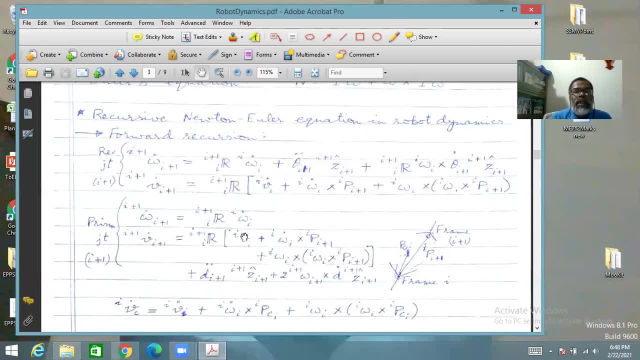 will have a lot of terms. First of all, the linear acceleration term: Linear acceleration of the previous joint origin, previous frame origin, plus the alpha cross r term, the direct angular acceleration term plus centripetal term. Now all these vectors to begin with. 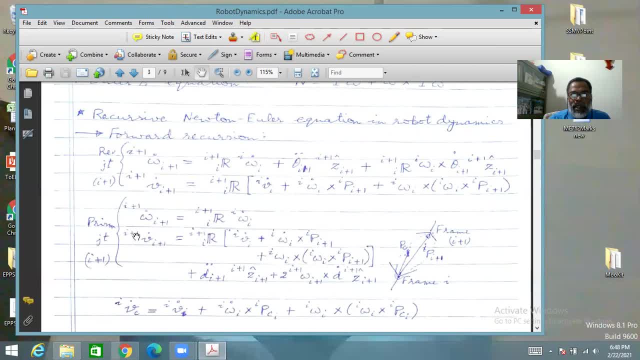 are available in i-th frame, So convert it into i plus 1-th frame, where the final result is asked for, Plus the two other terms, this is a direct linear acceleration term r double dot. Now this is a prismatic joint, So d double dot is the sliding acceleration at the joint into. 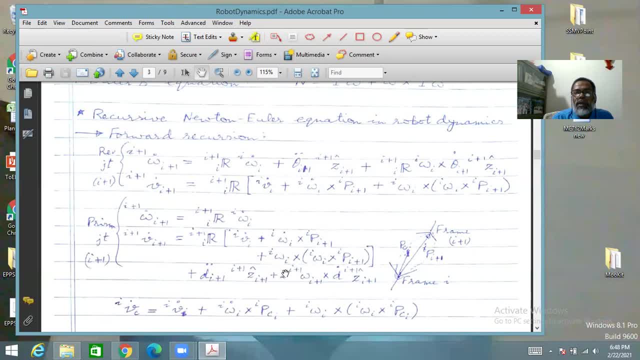 its unit vector, plus the Coriolis term, twice omega, cross, r dot. So here you see, all the five terms are there, The acceleration of the previous joint origin plus all the four terms. Now this is how the forward recursion in accelerations take place. And for writing: 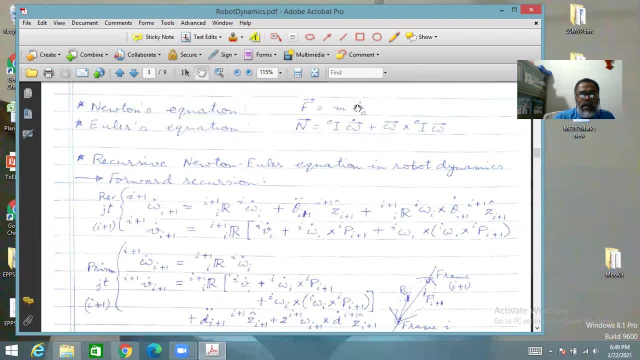 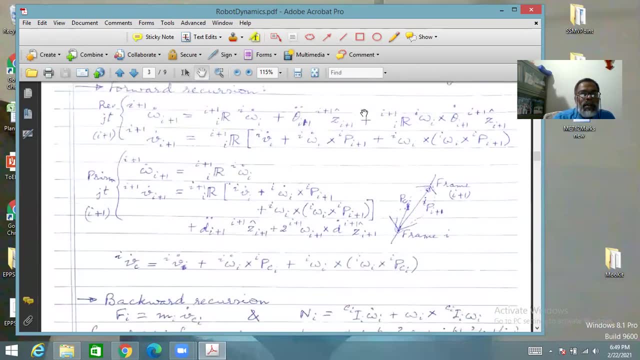 the dynamic equations later. basically, these equations, this equation, you will need the acceleration of the center of mass of every link. So find out that acceleration of the center of mass of the i-th link in its own frame. So the linear acceleration of the 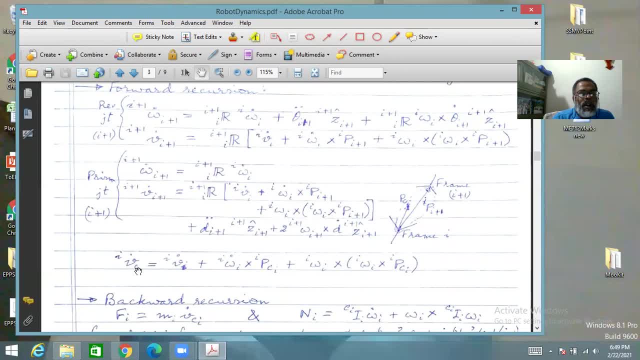 center of mass C of IS, link, The frame of that, the origin of the, the acceleration of the origin of the frame attached to that link. plus now it is a rigid body. so only the two rigid components, alpha cross r and omega cross, omega cross r, will come The r. 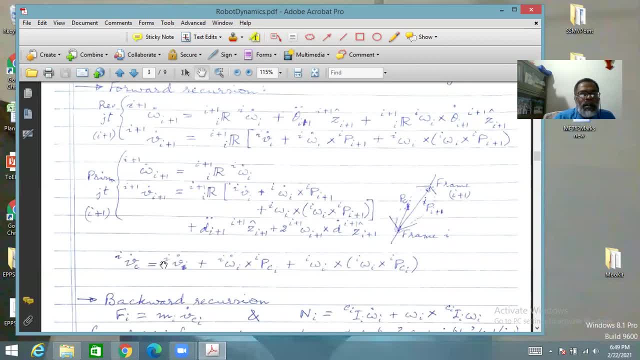 dot and r, double dot. related terms will not come okay. So this is the acceleration of the center of mass. Keep this in hand, okay. And the frame you have already got earlier. Now this recursively used for i equal to 0 to n, will give you acceleration of the linear. 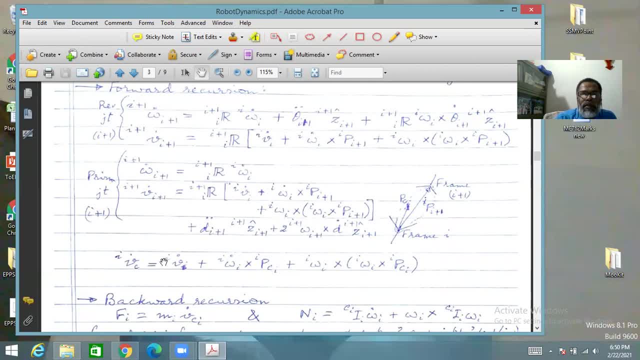 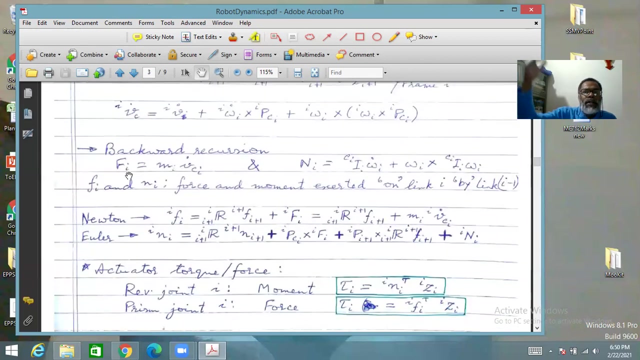 acceleration of each frame origin, linear acceleration of each center of mass and angular acceleration of each frame of reference on the way. okay, Okay, Now we start with the force. Now, as in static analysis, the force analysis takes place by backward recursion, right So, because the forces at the end are known, and forces 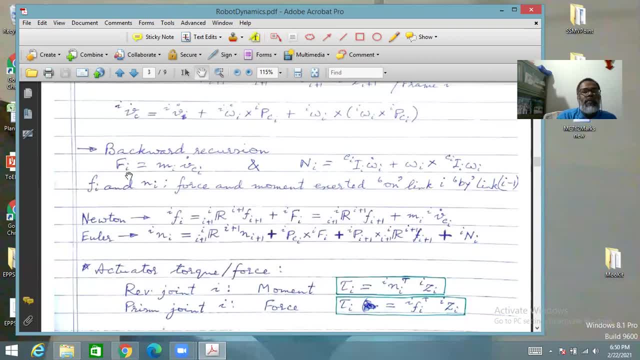 early at the earlier joints we will require: okay, So we apply the backward recursion on each of the links from n n minus 1, n minus 2 onwards. okay, And these two equations basically we write. So here we use the notation that F. 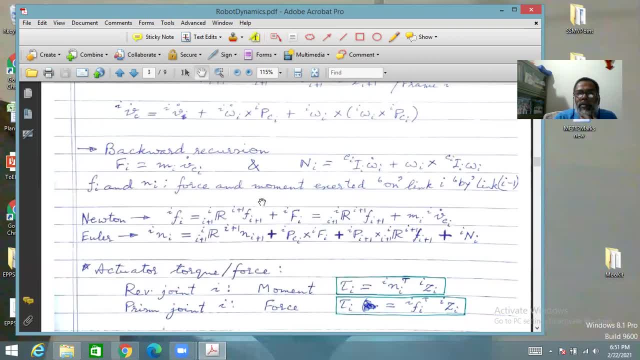 i and n. i are the force and moment exerted on link i by link i minus 1.. We had to use some notation. Either you could use this notation or you could use the force and moment exerted on link i by link i minus 1.. We had to use some notation. Either you could use this notation. or you could use the force and moment exerted on link i minus 1.. We had to do it 25 times. Now take this: This is is the moment exerted on link i by oftentimes i minus 1.. For instance, 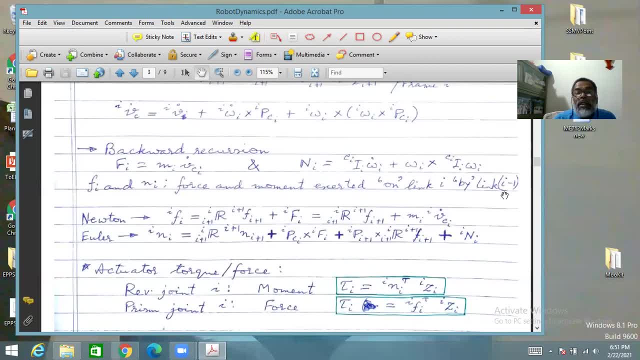 Ln i looks like this and Ln 2 looks like this. So it looks like Ln i is 1 up. This is the moment exerted on link i. Well, that is the moment exerted on years. Now f i is 1.. That is the moment exerted on link i by minus 1.. This is A, which means 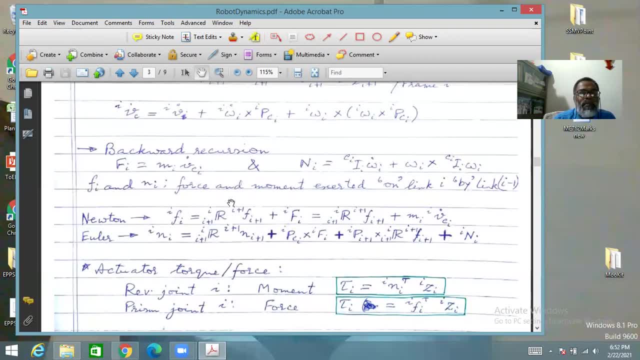 as long as I have the moment exerted on link i, I haven't chosen A, So now we have a particular and that will come in our equations, okay. So now, mass into acceleration of the center of mass, which we have got from here, is here. okay, That should be the sum total of all the forces applied. 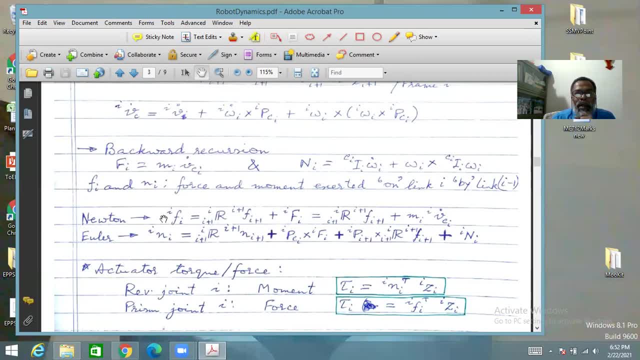 on link I: I minus 1 applies this force and I plus 1 applies the negative of this force, which is here. okay, So when you bring it on this side, because you see, this one is known for I equal to N, The forces applied on link N by N plus 1, which is environment: no link there. 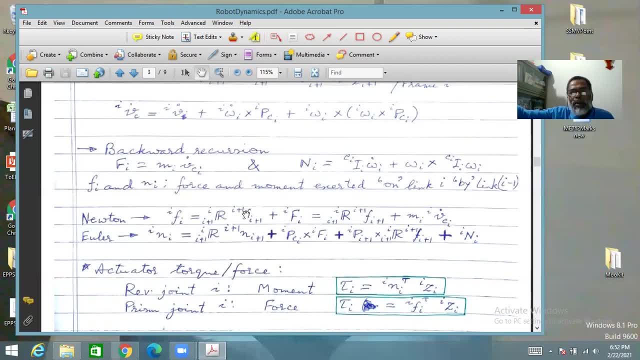 okay, is known, either 0 or whatever force, torque, whatever forces are coming that you know from the force sensor. So this is known, So the known thing, you bring it on this side and convert it into the proper basis. So from here you get I, F, I, that is, force applied on link I by link I minus 1, okay. 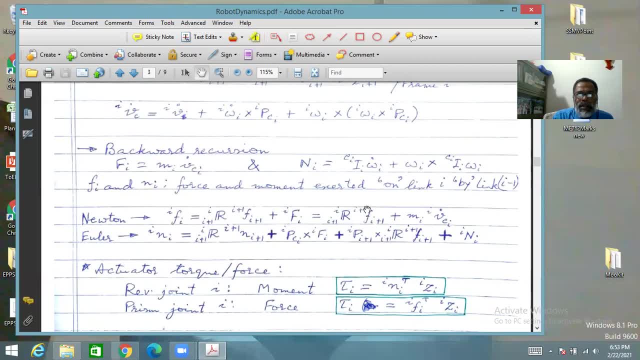 So okay, Here you insert this which you have got from the acceleration analysis by the forward recursion. So after the forward recursion ends, then you start the backward recursion. So this is from Newton's law, Newton's equation, And then for the moment you write the: 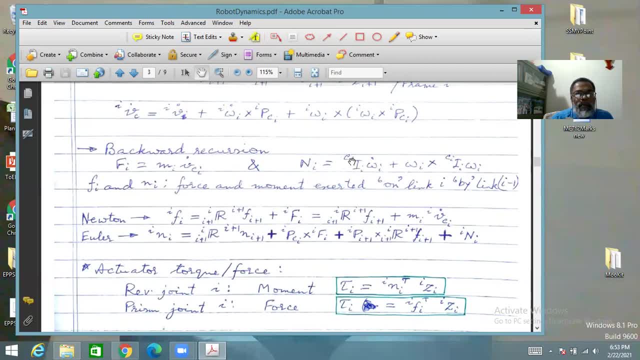 Euler's equation, and here keep in mind that this is for the pure rotational motion case, where the center of mass is not accelerated. okay, That is this. Now, if you take the moment about some other point, okay, if you take this moment about some other point, then to this you also have. 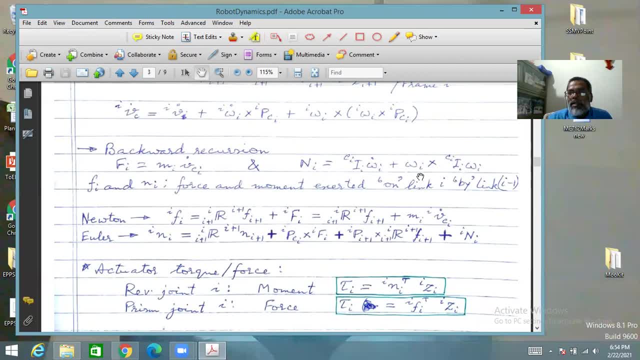 to add the moment contribution of the inertia force or the r cross mass into acceleration. Okay, so if you write the total moment on one side, that is, moment applied on link I by I minus 1, plus by 이 plus 1,, then negative of which is put here. okay, So it has been brought on this side Plus. 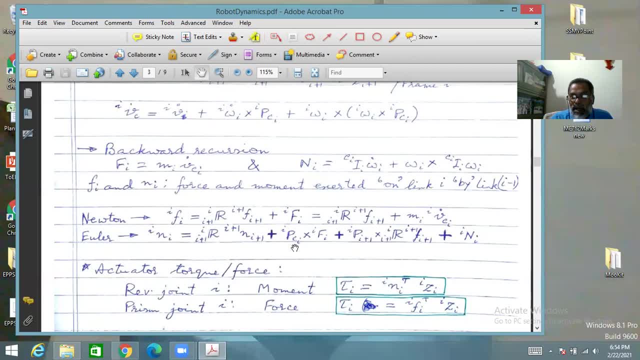 plus the r of the center of mass cross. this thing, okay, because since the moments are about some other point, so it also has to produce the moment of this. okay, so that is this plus the moment produced by the force from the next link, that is, this one, that is: 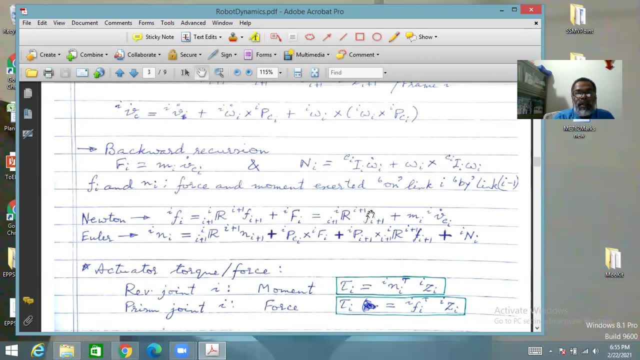 this force, moment of this force, and that is why the moment arm has been taken as the origin of the next frame of reference, plus the direct moment now, plus this, this is the result. actually, that is this. okay, so basically you say that the total moment which 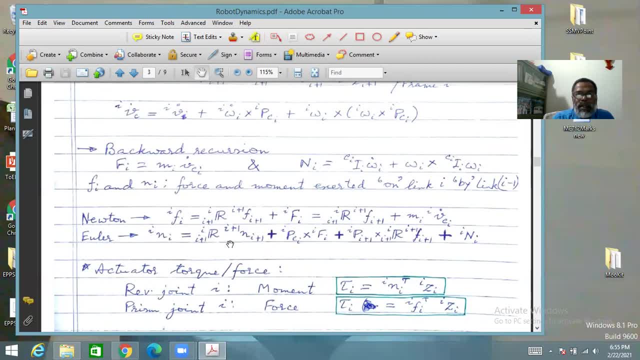 is this minus this, minus this, The moment of the force from the next joint, the present. the joint here doesn't have moment, because that is the origin of this moment. equation is equal to the moment to counter the angular inertia plus the moment to counter the linear inertia. which is this? okay, so? 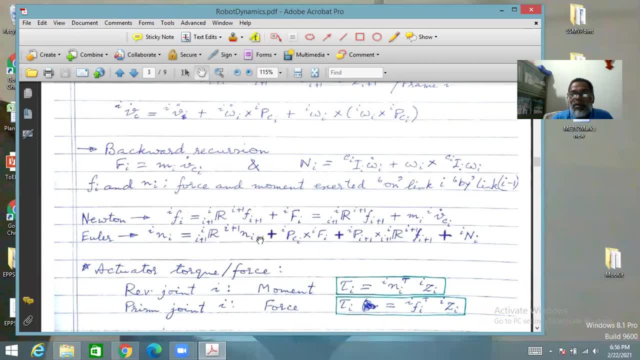 this entire thing. When you write and bring every other term which is known on this side, then you get this. okay, now, what these two equations give you, finally, what these two expressions give you. this give you the force exerted on link I by link I minus one. from here you can get. 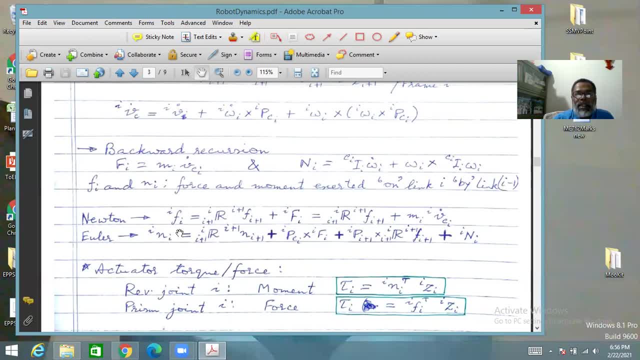 the actuator torque or actuator force of the IS joint. now, if the IS joint is revolute, then this entire Force is joint reaction and in this moment the Z component is the actuator torque. okay, so for revolute joint, you take the Z component of this. okay, basically the third component. 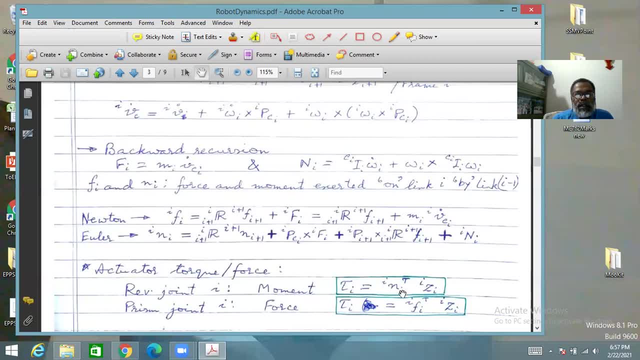 okay, because it is in the IS frame itself, the Z component. you take, that is this, the moment vector, dot, unit, vector along the Z direction, zero, zero, zero, zero, zero, zero one. okay. on the other hand, if the IS joint is prismatic, sliding joint, then the entire. 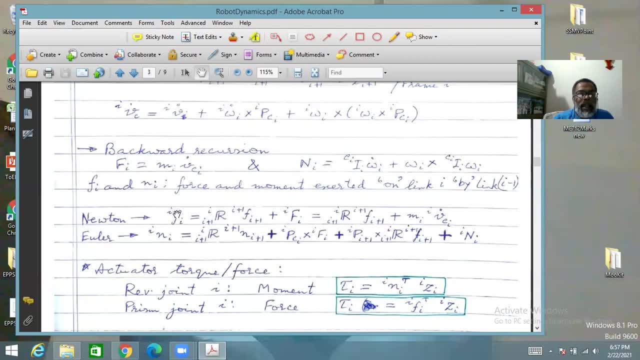 moment is joint reaction, and from the force you take the Z component and that is the actuator force. okay, so this is Newtonian error formulation. through the forward recursion you analyze the acceleration completely, Then by the backward regression, essentially by these two equations, you get all the forces. 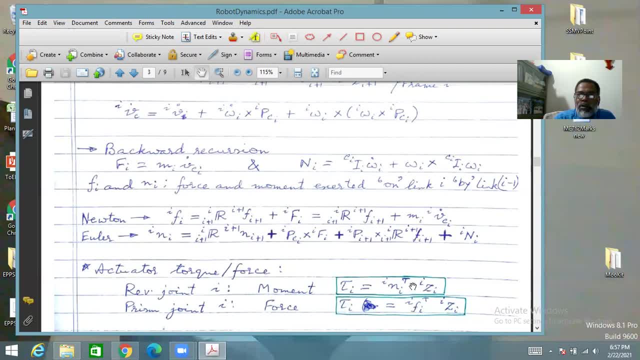 and vector forces and their appropriate components you pick up from here or from here, depending upon whether the joint is revolute or prismatic. so the actuator, efforts, moments or forces you get when the motion is known. okay, so this problem is known as inverse dynamics. 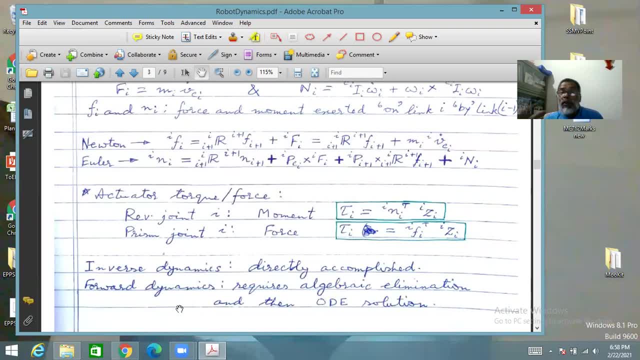 and that is directly accomplished from this. If you want to do forward dynamics, that is, knowing the actuator torques and actuator forces, if you want to find out the resulting motion, then you will need to first get these equations from there, eliminate all the constraint forces algebraically. that elimination is: 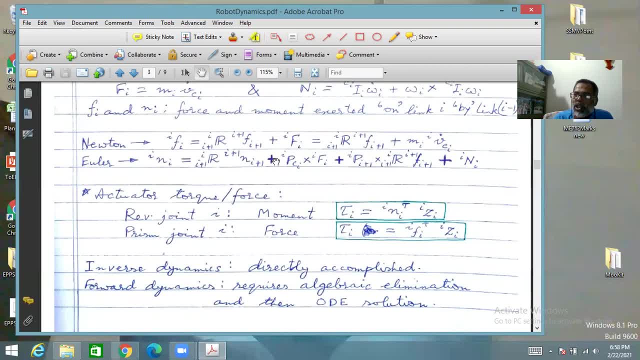 very simple but lengthy, because for each body you will have six equations from here: three force equations, three moment equations and out of each force-moment combination, that is six quantities. six out of the six quantities, five are constraint forces and 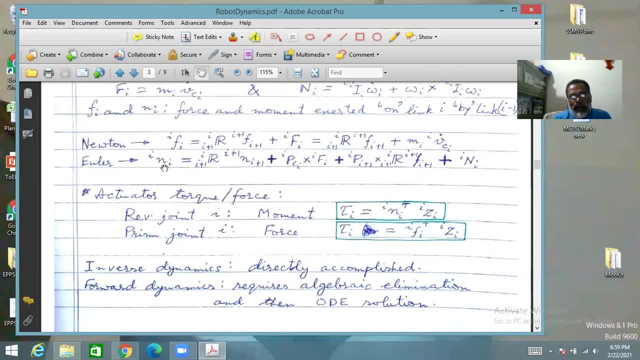 moments, only one is actuator torque or actuator force. so those five constraint forces and moments You have to eliminate, okay, so out of six equations you need to eliminate five, five unknowns. okay, so when all those unknown constraint forces which you don't need and